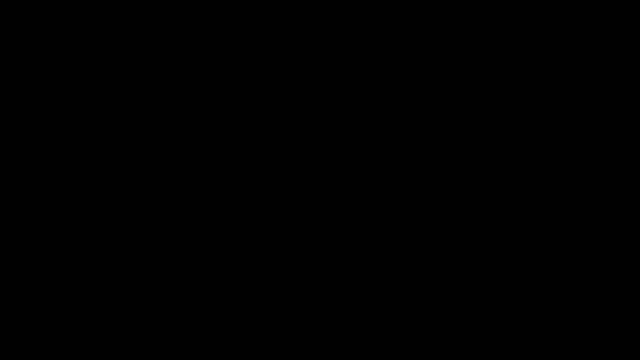 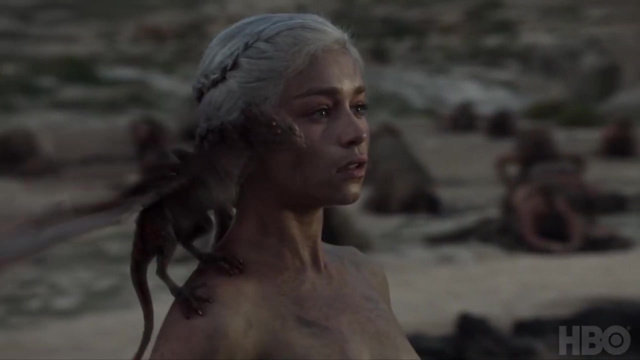 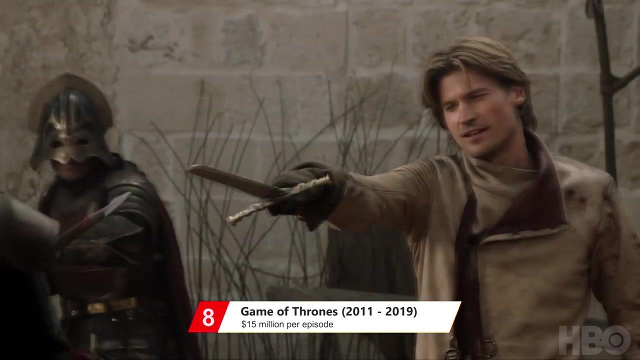 Golden Globe and Primetime Emmy awards. Number 8.. Game of Thrones: Fantasy drama TV series produced by HBO based on George RR Martin's novels. The HBO series had a budget of 15 million dollars per episode, with a total budget of 10 million dollars per episode. 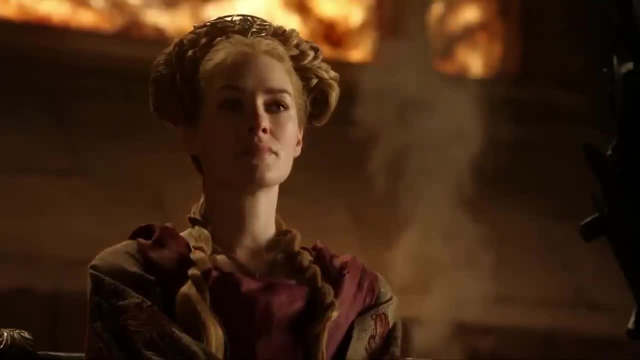 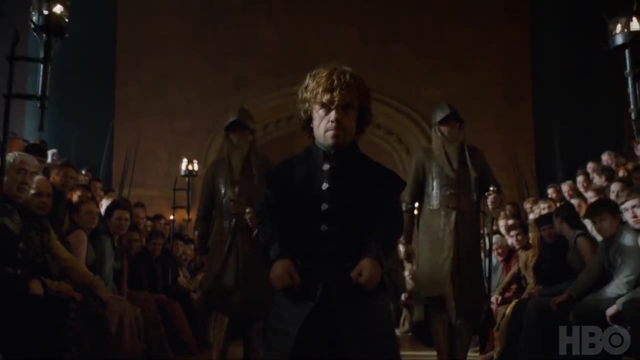 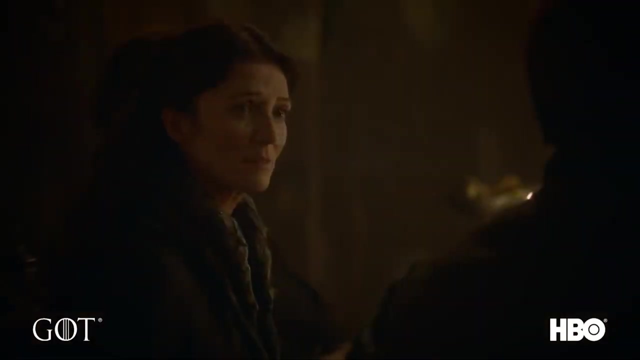 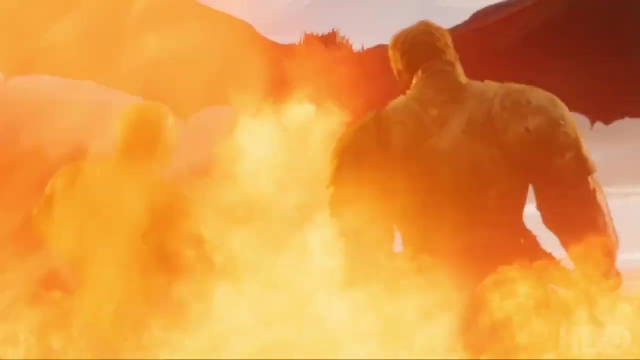 The show takes place in the fictional continent of Westeros, where noble families fight for control of the Iron Throne. The series is known for its complex plot, political intrigue, shocking twists and turns, large-scale battle scenes and, of course, dragons. It was praised for its performances. 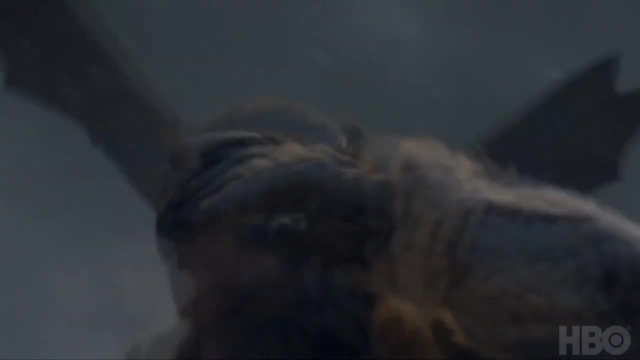 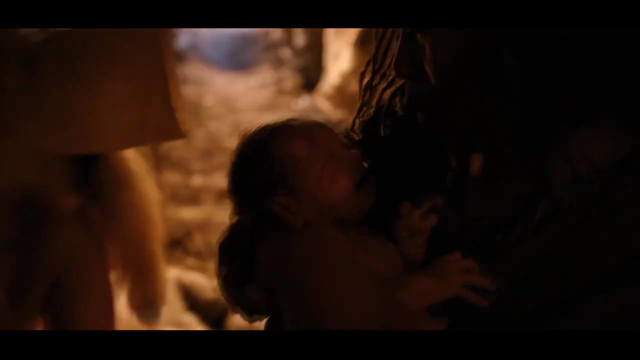 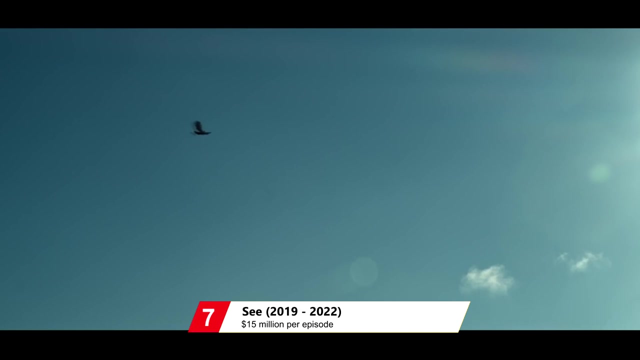 direction and production values, and it became one of the most popular shows in the world. It was also one of the most popular and critically acclaimed TV shows in the world, Number 7. Sea. It's a post-apocalyptic science fiction television series that takes place in a distant future. 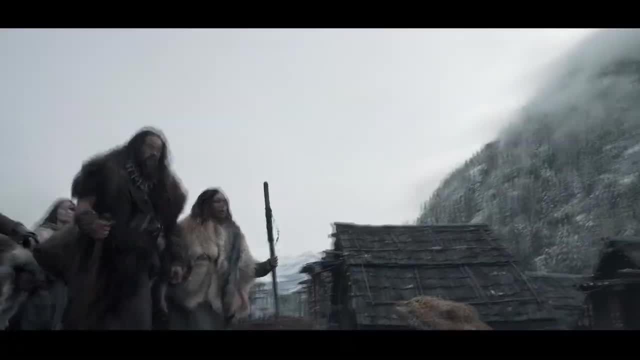 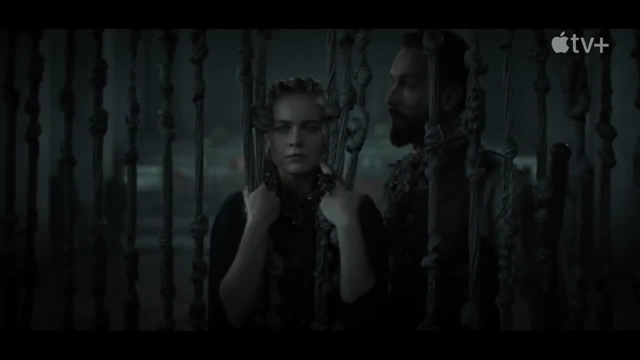 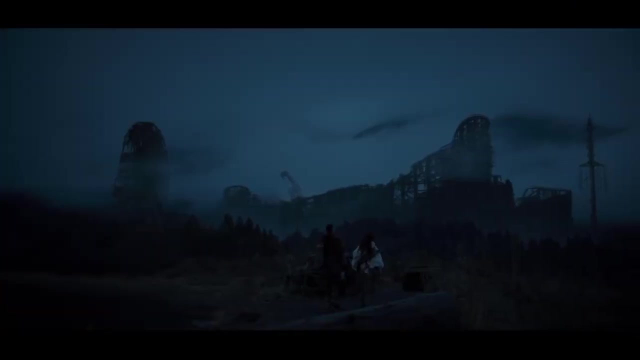 where humanity has lost the ability to see and they have to adapt to a new way of life. The show follows a warrior, chief, Baba Vaas, and his family as they navigate this new world and protect the tribe against a powerful enemy. The series first premiered in 2019 and features a 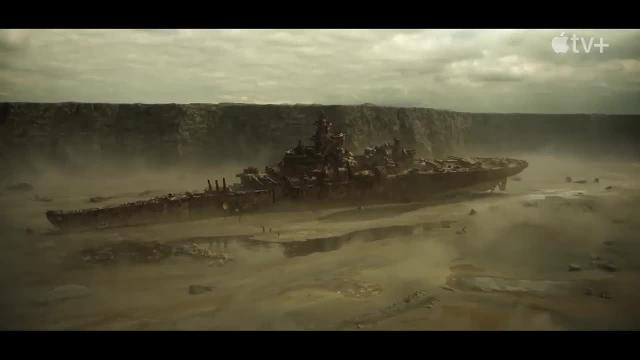 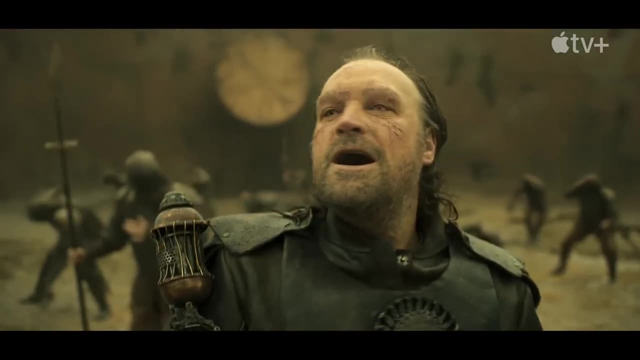 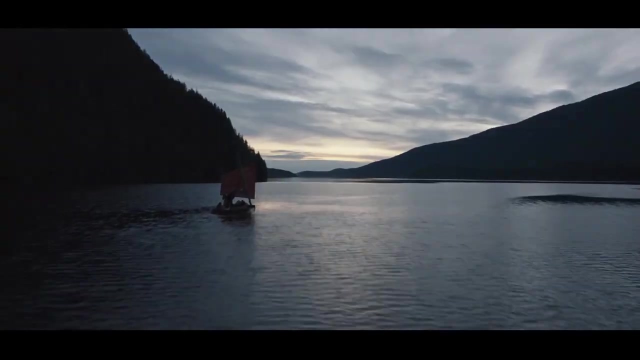 talented cast of actors such as Jason Momoa playing the lead role as Baba Vaas. The budget of 15 million dollars per episode shows with its visually stunning production, and the show is known for its unique premise and its exploration of the power of a family and community in the face of 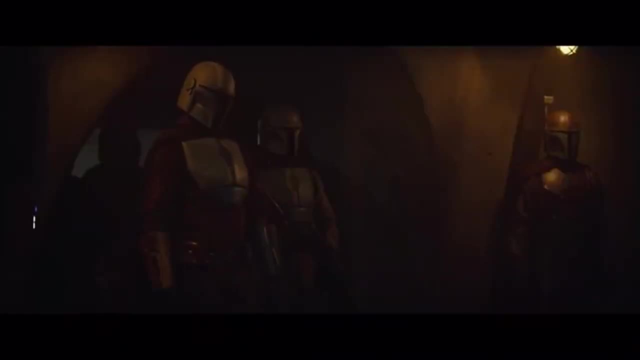 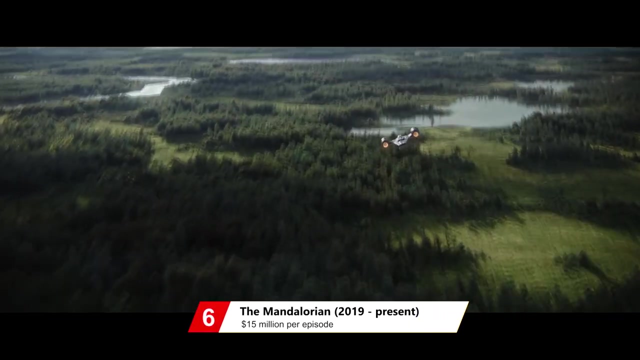 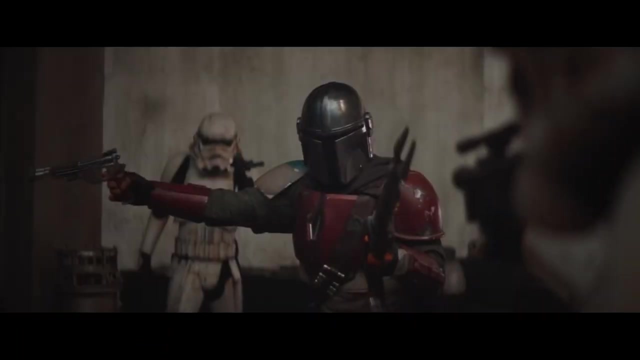 adversity. This is the way. This is the way. This is the way. Number 6. The Mandalorian. Created by Jon Favreau for Disney Plus and a budget of 50 million dollars per episode, the series is set in the Star Wars universe and follows the story of a lone Mandalorian. 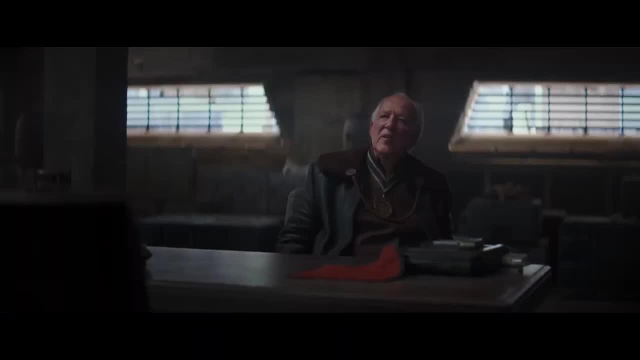 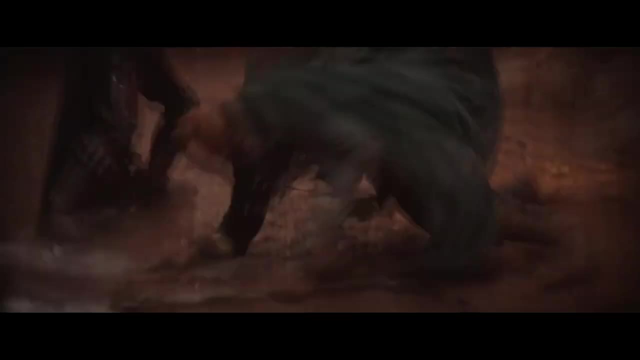 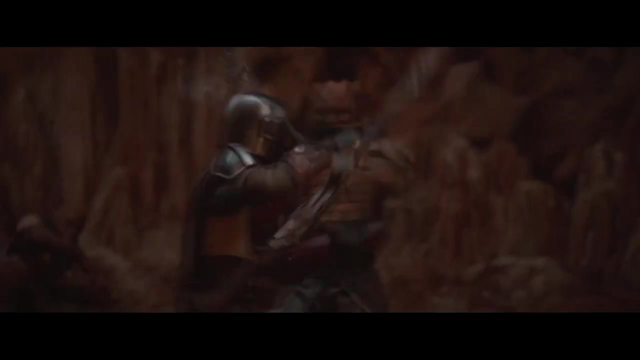 bounty hunter, Din Djarin, As he undertakes various dangerous missions while trying to find a way to return a child of the same species as the iconic character Yoda to its people. The show premiered in 2019 and featured Pedro Pascal as the leading role of the Mandalorian. 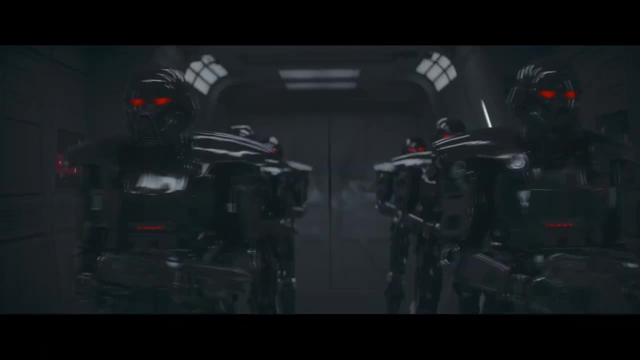 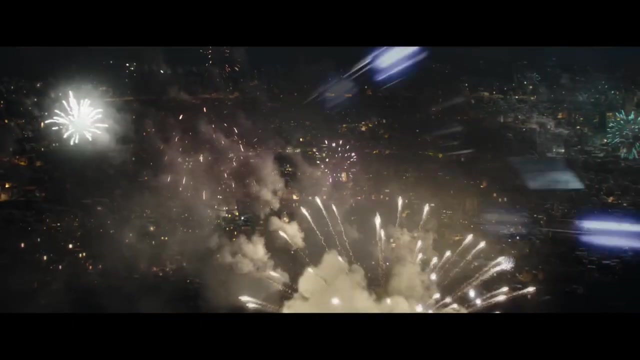 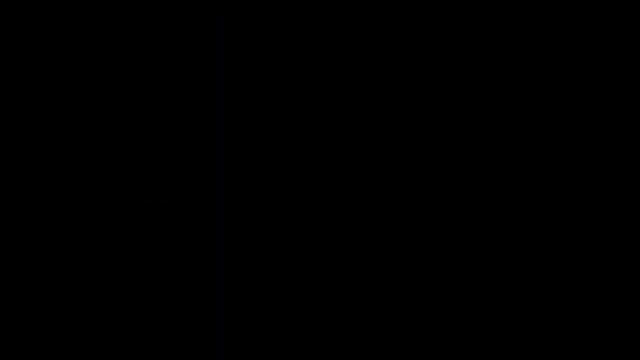 The show is known for its visually stunning production, its action packed story and its exploration of the Star Wars universe that so many people love. It has received widespread critical acclaim and has won multiple awards. Number 5. The Pacific: Number 5. The Pacific: A war drama. television miniseries created by Peter Parker and Eric 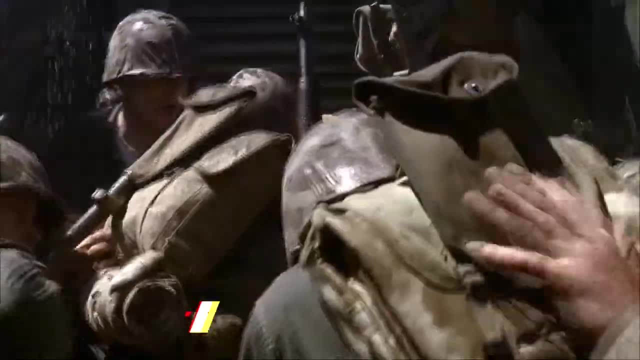 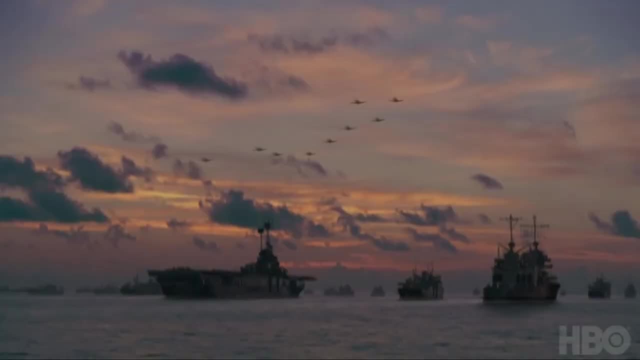 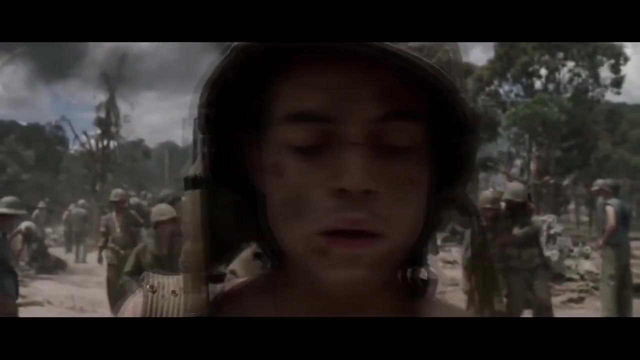 was created by Steven Spielberg, Tom Hanks and Gary Goldsman for HBO. The series is based on the experiences of United States Marines in the Pacific Theater of World War II, and it follows the stories of three US Marines from their boot camp training to the Battle of Palu. 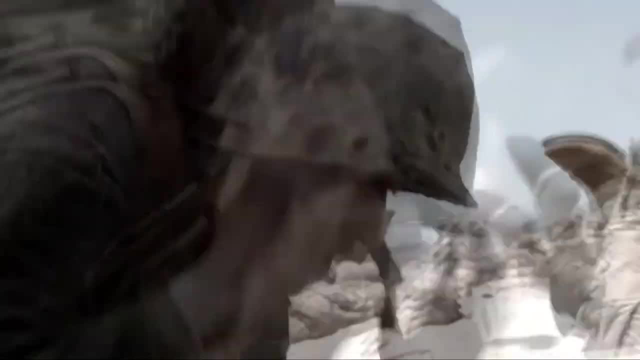 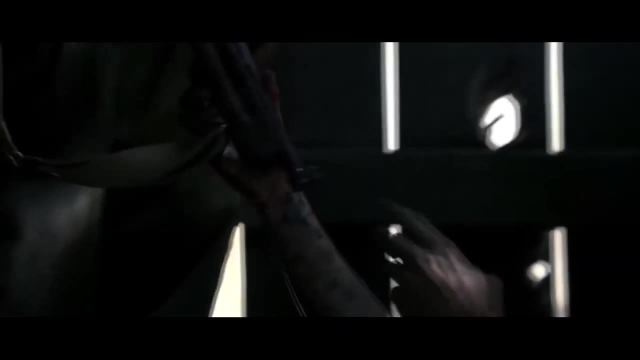 The series premiered in 2010 and has 10 episodes in total and with a budget of 20 million dollars per episode. the series is known for its realistic and graphic portrayal of war. It's also known for their attention to historical accuracy and its exploration of the psychological 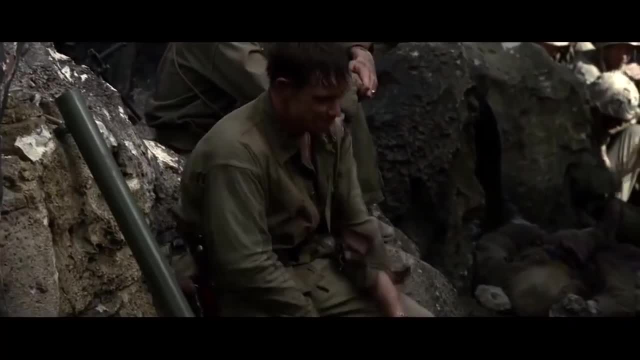 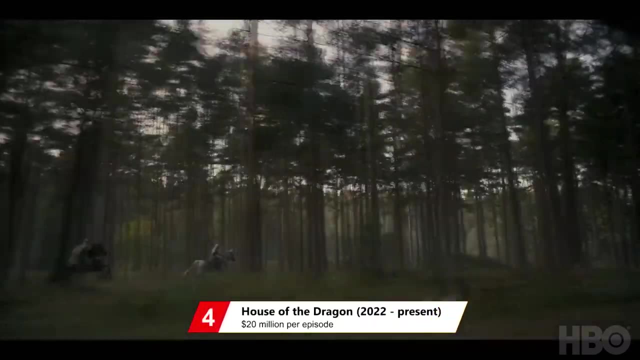 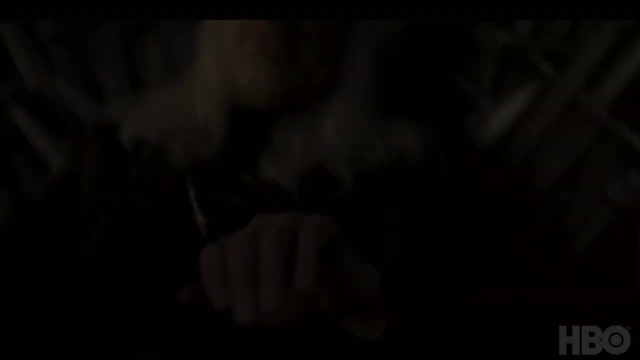 effects of war on soldiers. The series has won multiple awards. Number 4. House of the Dragon is a historical fantasy television series created by George R R Martin and Ryan Condal for HBO. The series is based on Martin's book Fire and Fire. 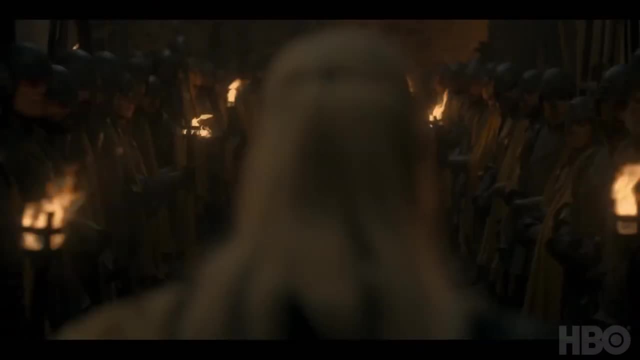 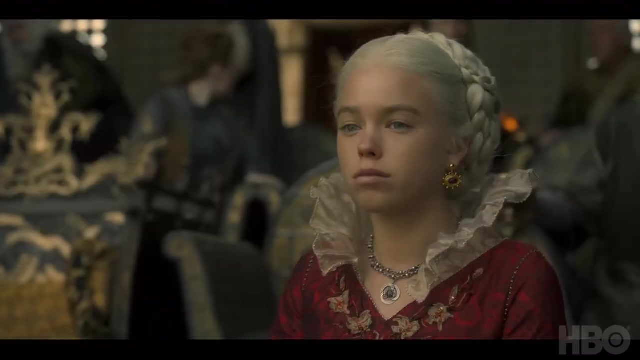 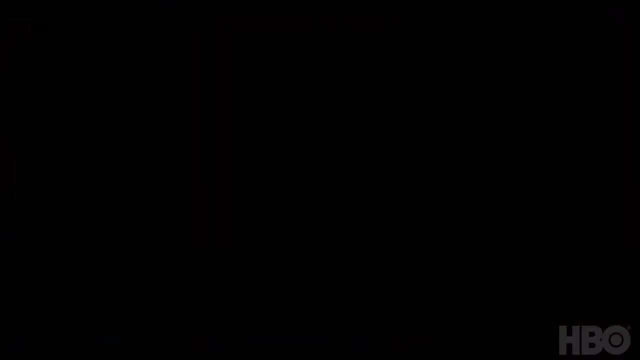 It tells the story of House Targaryen, a family of dragonlords who use the dragons to conquer the Seven Kingdoms of Westeros. The show takes place several centuries before the events of Game of Thrones and it depicts the Dance of the Dragons- a Targaryen civil war. 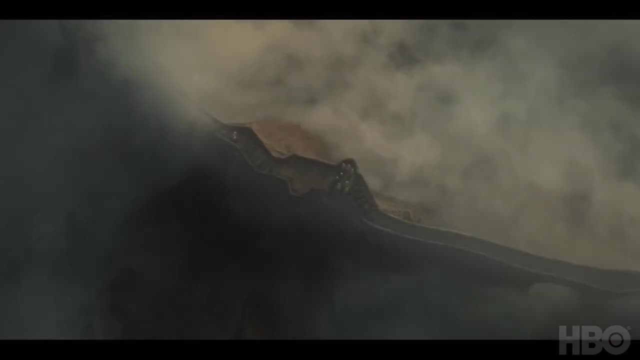 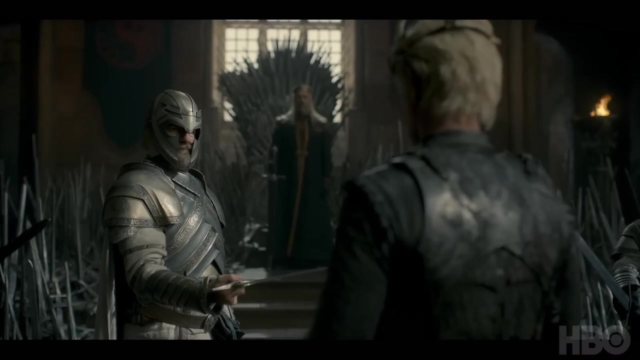 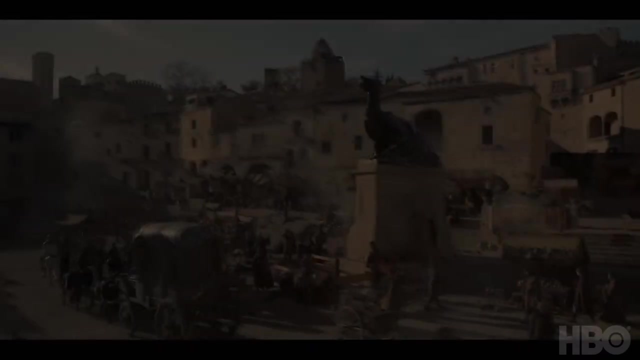 With a budget of 20 million dollars per episode. the show debuted in 2022 and features a talented cast of actors, including prominent characters from the Targaryen family. The show is known for its visually stunning production, complex political story and. 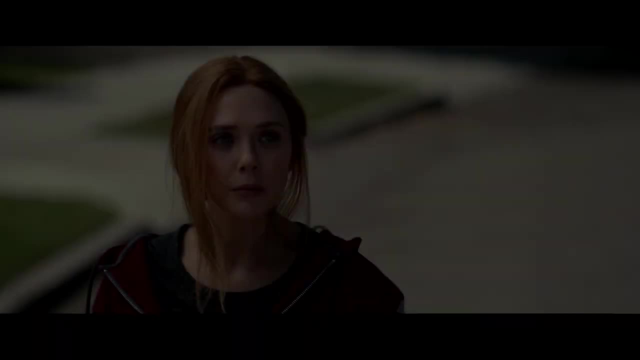 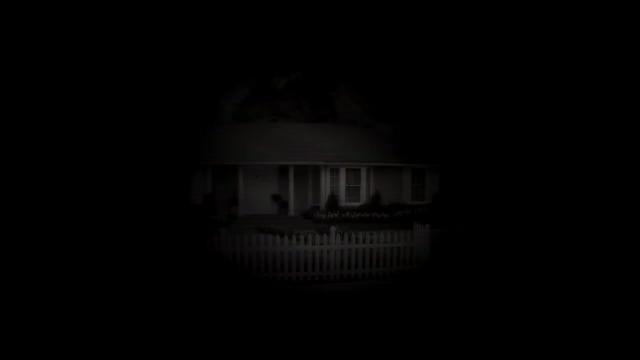 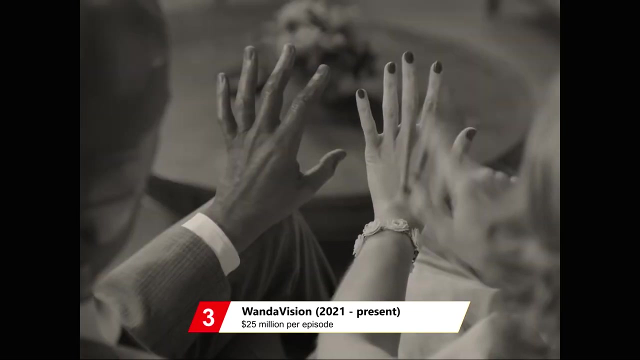 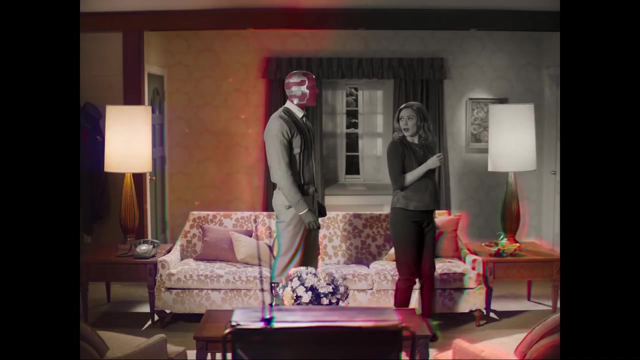 exploration of the human condition. Number 3.. Wandavision is a superhero television series created by Disney Plus by Jack Schafer. The show is based on a true story. The show is based on a true story. The show is set in the Marvel Cinematic Universe and follows the characters Wanda Maximoff. 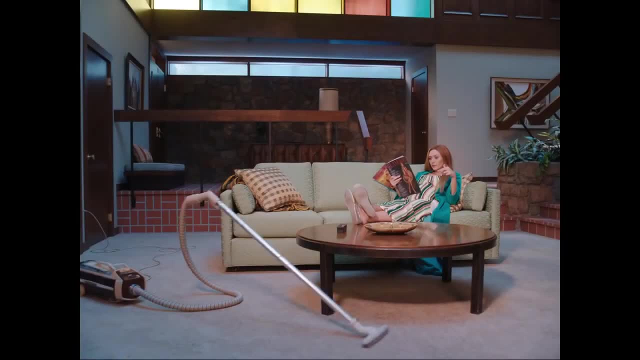 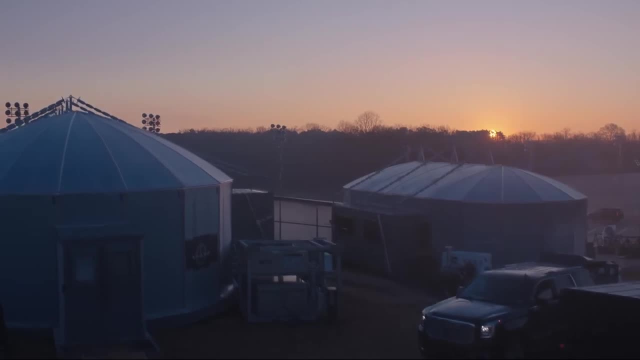 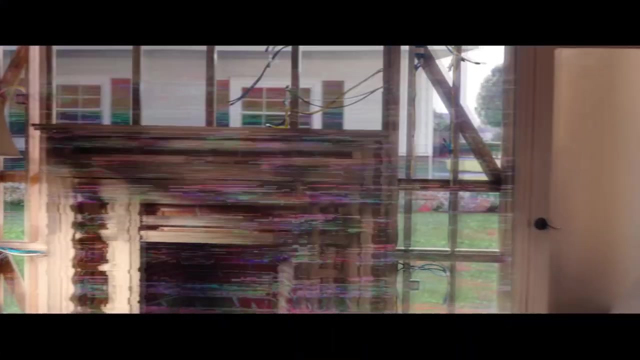 and Vision as they navigate through various different eras of sitcom, setting Together with a lot of the popular MCU TV shows. Wandavision has a budget of 25 million dollars per episode. The show premiered in January 2021 and had nine episodes in total. 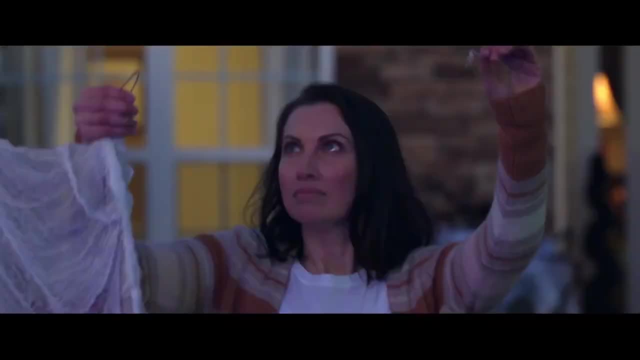 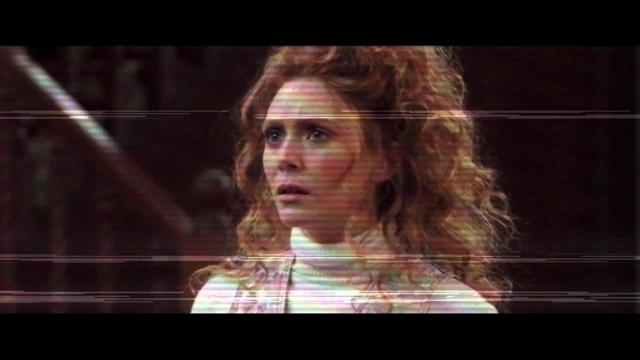 The show features a talented cast with Elizabeth Olsen and Paul Bettany playing the lead roles as Wanda and Vision. The series is known for its unique blend of classic sitcoms and the Marvel Cinematic Universe, its blend of humor and drama and its exploration of the character's emotional 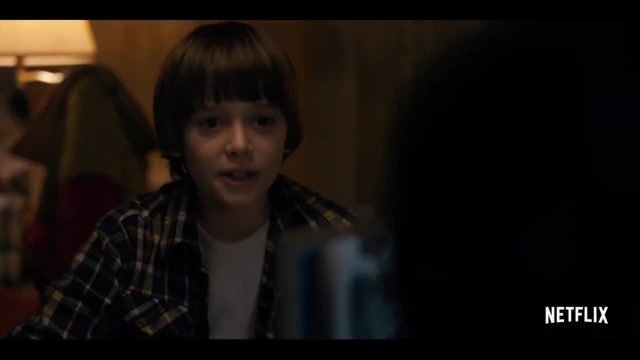 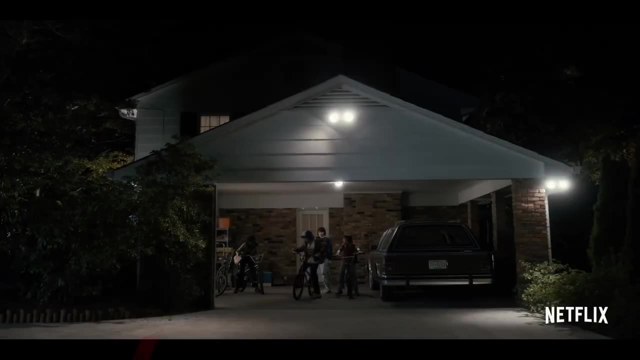 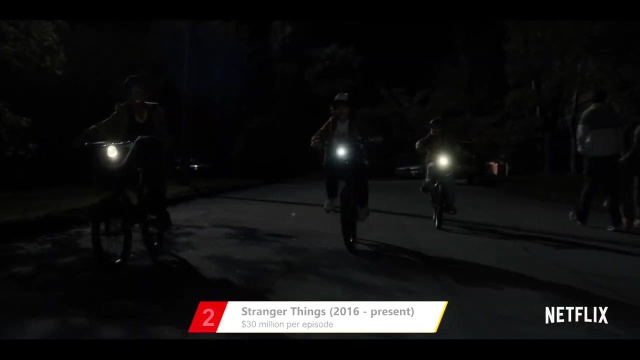 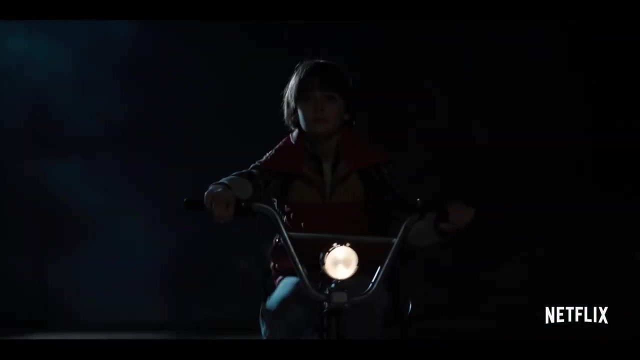 arc Number 2.. Stranger Things, The Netflix series, has a reported budget of 30 million dollars per episode, with a total budget of over 80 million dollars for its first season alone. Stranger Things is a science fiction horror television series created by the Duffer Brothers. 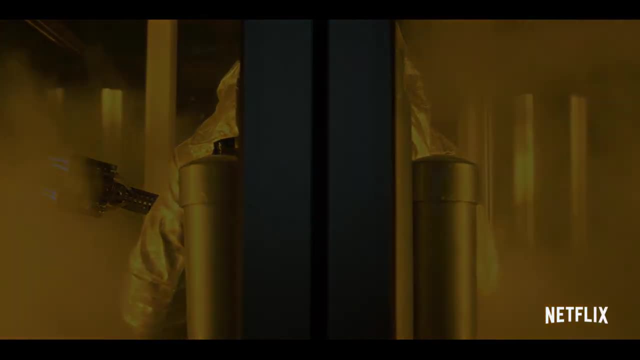 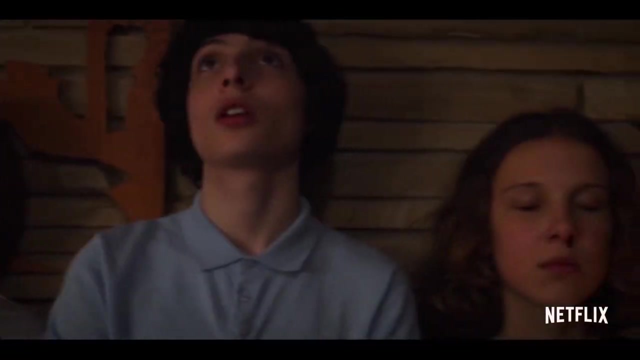 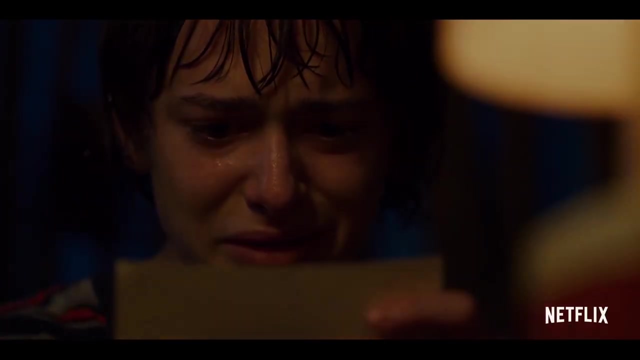 for Netflix. The show is set in the fictional town of Hawkins, Indiana, in the 1980s and follows a group of friends as they uncover supernatural and paranormal events happening in their town, including the disappearance of one of their own and secret government experiments. 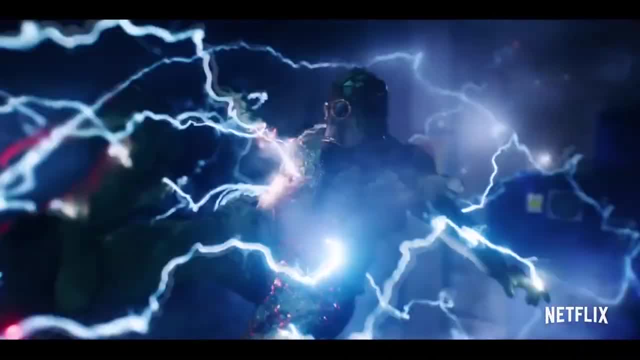 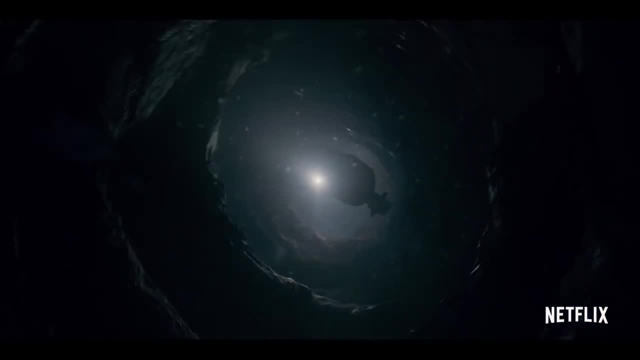 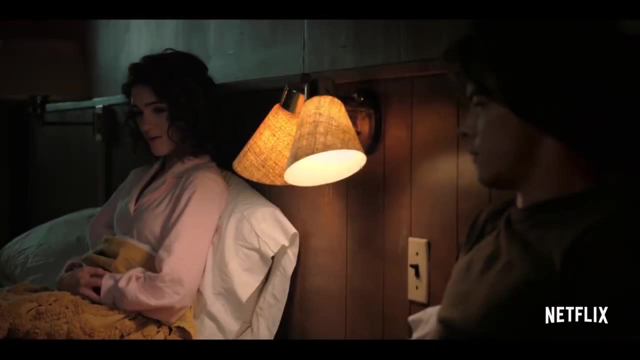 The show first premiered in 2016 and has four seasons to date. The show first premiered in 2016 and the series is known for its nostalgic 80s references, its suspenseful plot and its strong performances. It has been widely popular and critically acclaimed and has won multiple awards, including Primetime Emmy Awards, Number 3.. WandaVision. The show premiered in 2016 and has four seasons to date. The show first premiered in 2016 and the series is known for its nostalgic 80s references, its suspenseful plot and its strong performances. 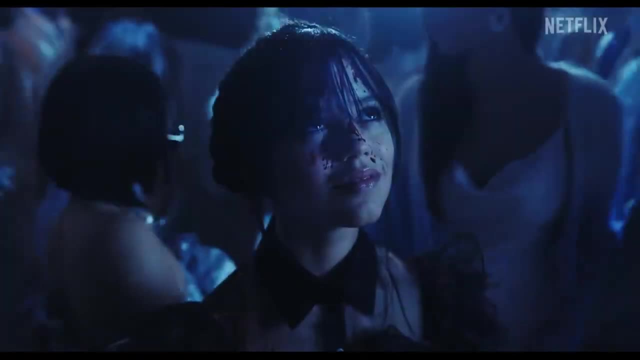 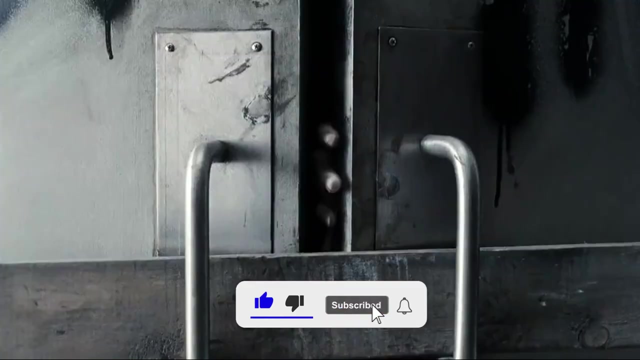 The show came out on display in 2011 and was film entire 2017 and again in 2017.. We have been going through nine of the most expensive Poker screenings of the year after it came out and the Show once again is given a활goömico award. 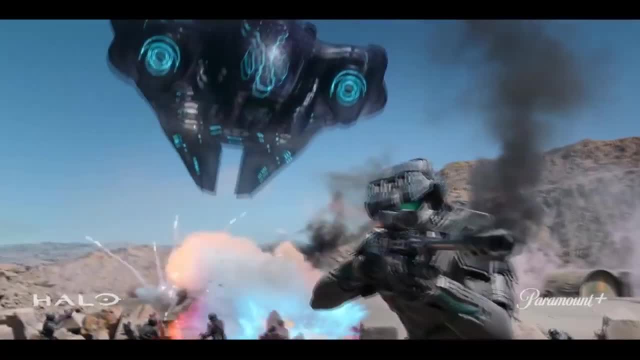 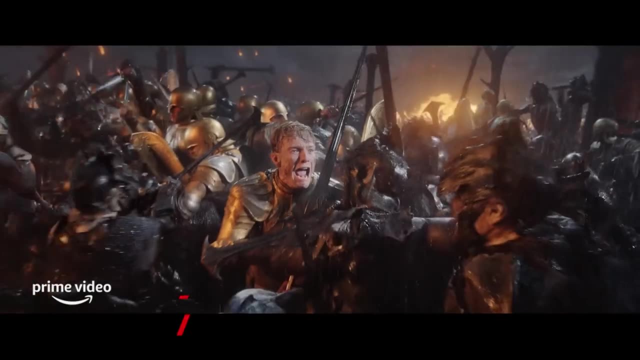 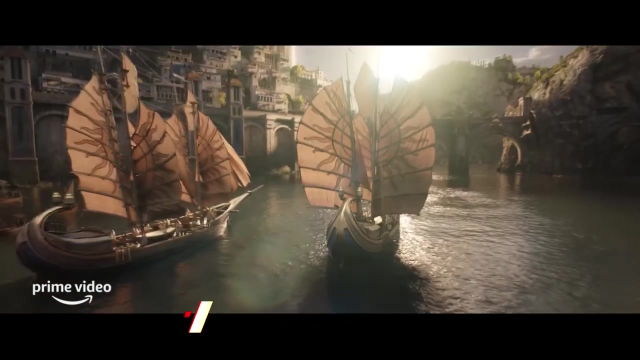 • PatПunt 1. The Rings of Power: The film package. These films- plotline designed, directed and performed by Marc ARsola and Megan Fleish, Have slightly different screenings at the. In 2001, JRR Tolkien's popular trilogy became one of the film industry's biggest. commercial and critical successes. The production was also one of the most expensive of all time, so it's not surprising that the big guns are being brought out and no expenses is being spared when creating the TV show that explores stories outside of Lord of the Rings and The Hobbit. For the first season alone is estimated to be around $465 million, and the show's budget is $58.1 million per episode, And that is excluded for the events of The Hobbit- and the plot revolves around the forging of the 19 rings by elves under the influence of Sif.